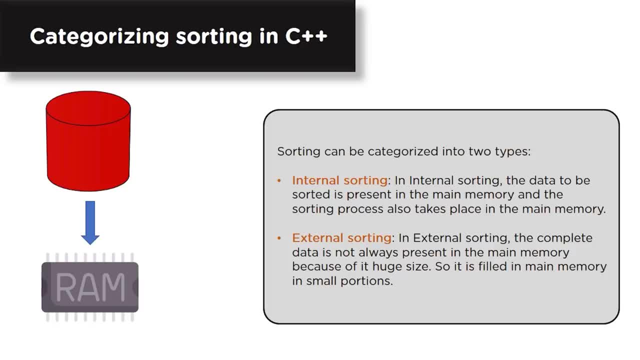 the data to be sorted is present in the main memory, and the process of sorting will also take place in the main memory itself, While in case of external sorting the data is not always present in the main memory because the data is large, So data is filled in the 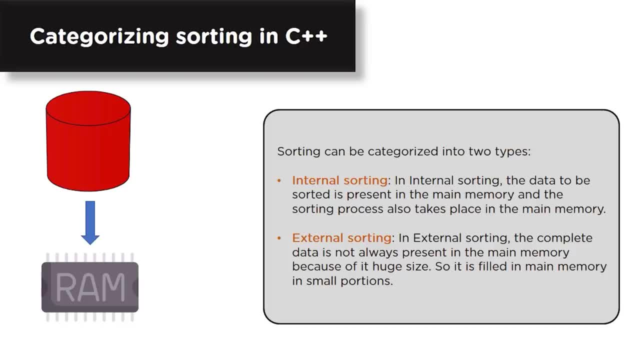 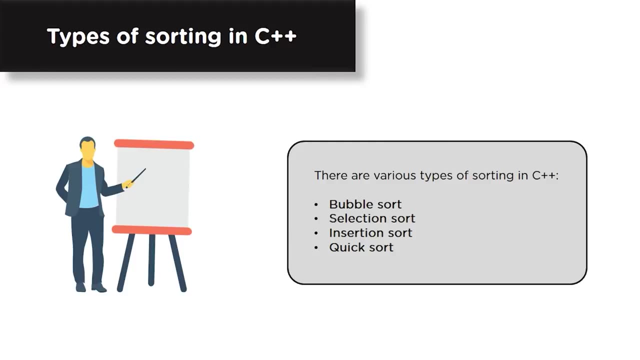 main memory in small portions. So this is the difference between internal sorting and external sorting. So let's understand these. Now, coming to types of sorting in C++, There are various types of sorting in C++ that are bubble sort, selection sort, insertion sort and quick sort. So let's start with bubble. 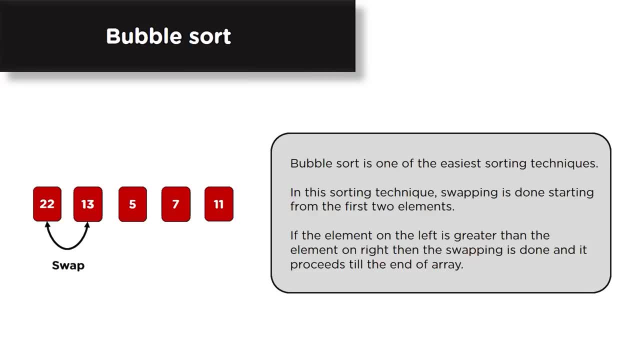 sort. Bubble sort is one of the easiest sorting techniques in C++. In this technique, the comparisons are done starting from the first point. So let's start with bubble sort. Bubble sort is one of the easiest sorting techniques in C++. In this technique, the comparisons are: 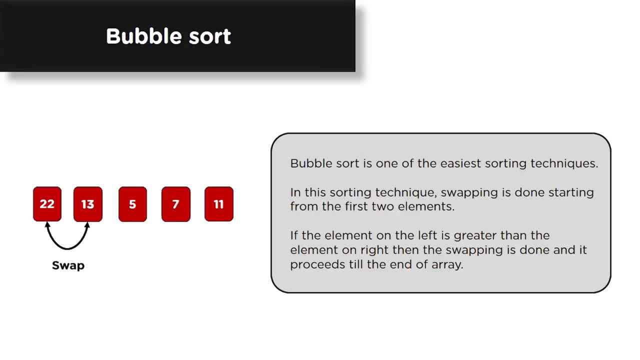 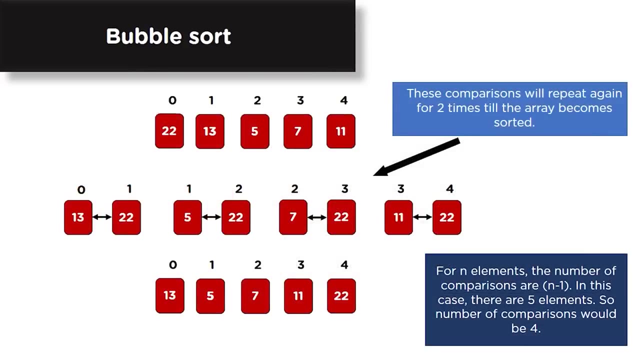 made after swapping two elements. The adjacent elements are compared. if the element on the left is greater than the element in the right, then the swapping is done and it will proceed till the end of the array. So first the comparison will start from the first two elements that. 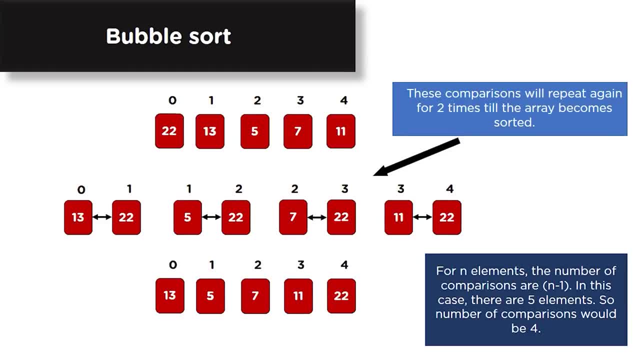 are 22 and 13.. And as we know that 22 on the left is greater than 13. So we will swap these elements and make them 13 on the right, As we have learned that the elements on the left are greater than the elements in the left, So the switches between the two elements are: 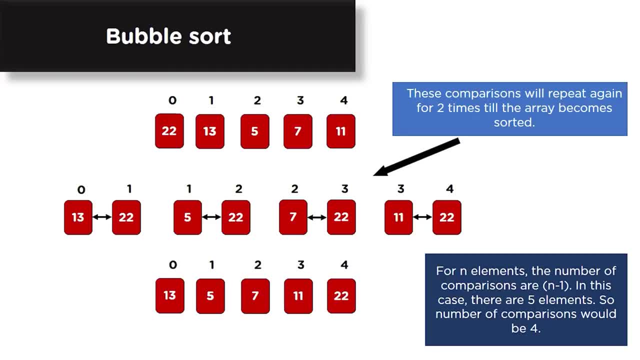 13 on the left and 22 on the right. Now it became 13,, 22,, 5,, 7,, 11.. So now we will compare 22, which is at index 1, with 5, that is at index 2, and as 22 is greater than 5, we will swap. 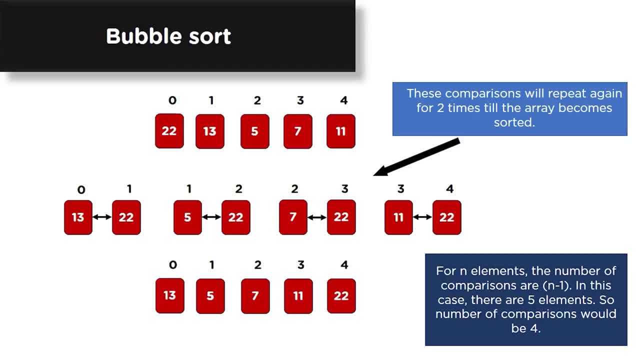 these elements as well, Then again we will compare it with the next element, and if 22 is greater than that element as well, then we will swap them as well. So in this way, round 1 of comparison is complete, as one of the element reached its actual position. Two: 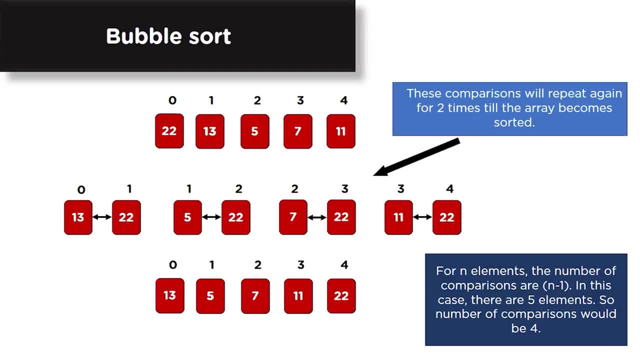 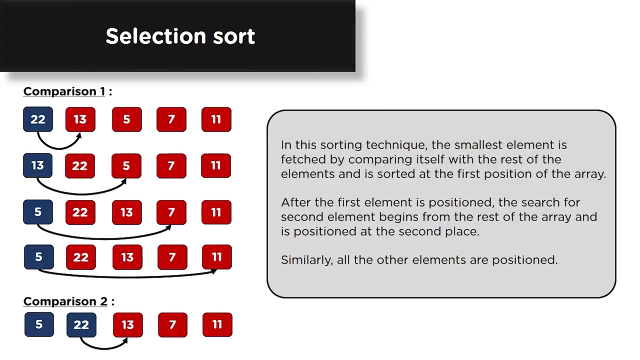 more rounds of the comparisons will occur till the array becomes sorted. It is because for n elements the number of comparison are n-1. So number of comparisons here would be 3, as the elements are 4 in numbers. Now coming to selection sort. In this selection sort technique the smallest element is fetched. 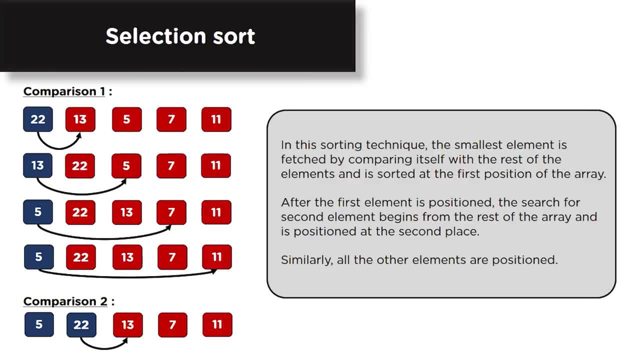 by comparing itself with the rest of the elements and is sorted at the first position of the array. Once the first element is sorted, the search for second minimum element begins from the rest of the array and is positioned at the second place. Similarly, one by one, all the elements are positioned like this. So this is selection sort Now. 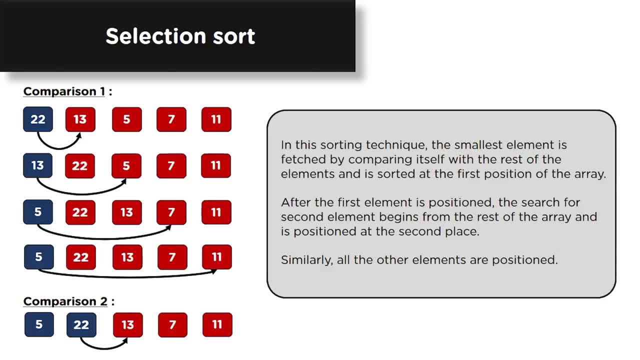 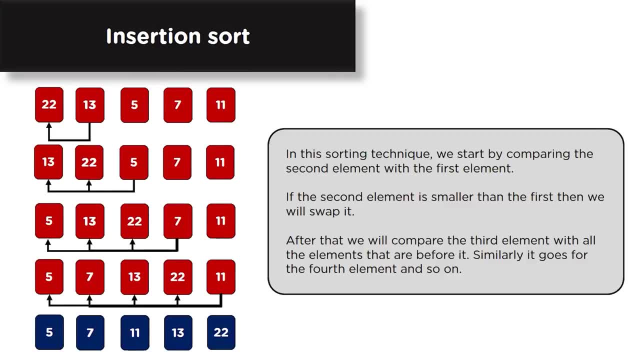 moving to insertion sort technique. In this sorting technique, the elements are sorted by comparing the second element with the first element. If the second element is smaller than the first, then we will swap it. After that, we will compare the third element with all the elements that are before it. Similarly, it goes for the fourth element, and so on Once. 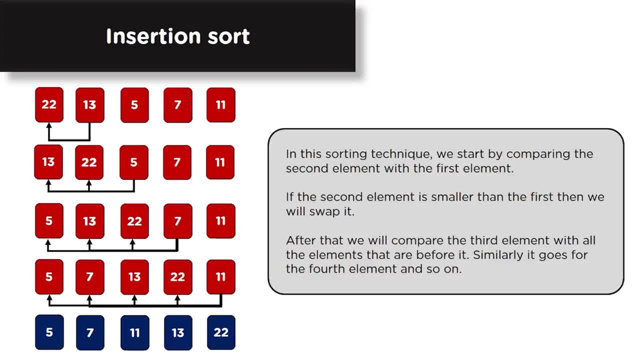 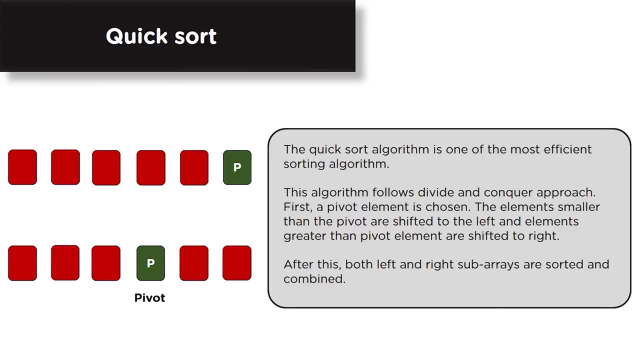 all the comparisons are done, the elements becomes sorted, as we can see in the figure. This was insertion sort technique. Next is quick sort technique or quick sort algorithm. Quick sort algorithm is one of the most widely used algorithm and the most efficient sorting algorithm. 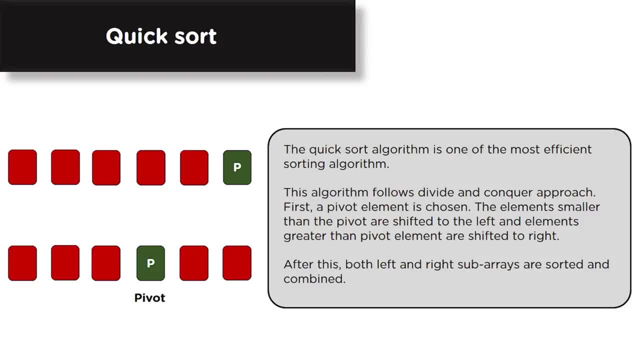 The quick sort algorithm follows a divide and conquer approach. In this approach, a pivot element is selected and the array is partitioned into two halves on the basis of this pivot element. The elements that are smaller than the pivot element are shifted to the left side of it, and elements greater than the pivot element are shifted to the right side of it. 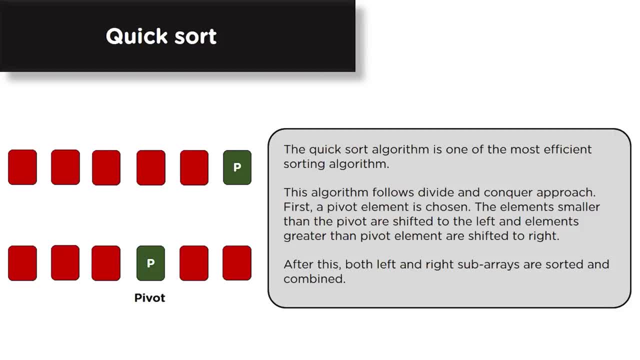 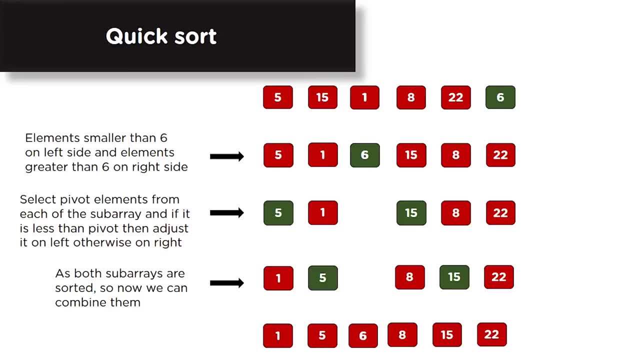 After this, both the left and right sub-arrays are sorted and combined. This is called a quick sort algorithm. The quick sort algorithm follows a divide and conquer approach. In this approach, a pivot sorted and combined. For example, let's suppose we have 6 elements, 5,, 15,, 1,, 8,, 22 and 6 and we 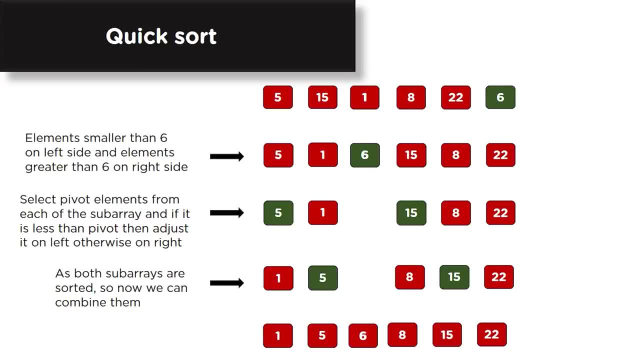 want to sort them using quicksort. So first of all we will select any pivot element, let's say 6.. Now we will divide the array to two sub-arrays based on the pivot element, in such a way that the elements smaller than the pivot element are on the left and the elements greater than the pivot 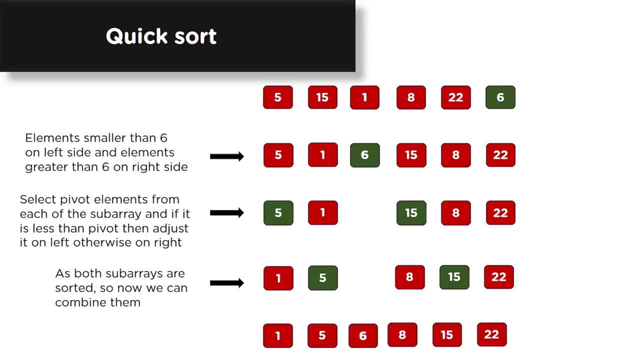 element are on the right. As you can see in the figure, elements smaller than 6 are on the left and elements greater than 6 are on the right. Now we will sort both of these sub-arrays separately. We will select a pivot element from each of the sub-array, Like we can see. 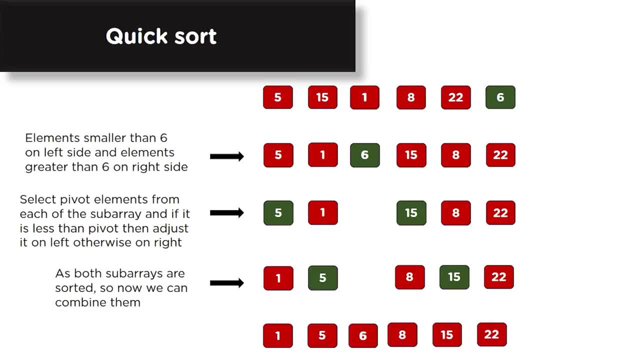 from the first sub-array. we have selected 5, and the sub-array is on the left. Now we will sort both of these sub-arrays separately. second subarray: we have selected 15.. Similarly, if the element is less than the pivot element. 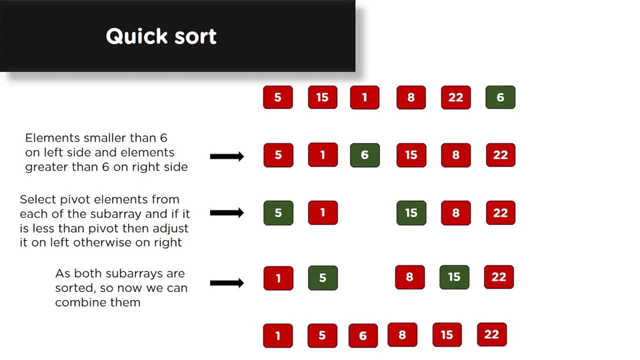 then adjust it on the left, otherwise on the right. By doing this, both the subarrays will become sorted and now we can combine them to become a complete sorted array. So this is how quick sort algorithm works. So, as we have understood about the sorting technique, 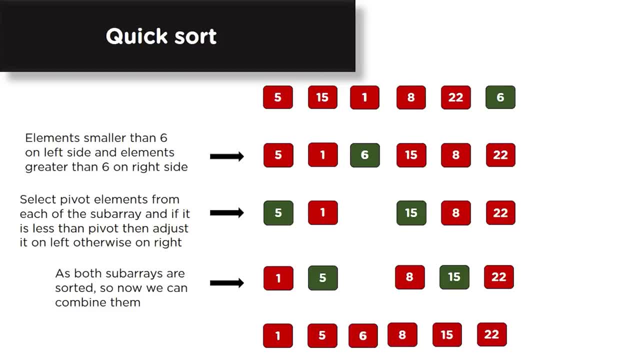 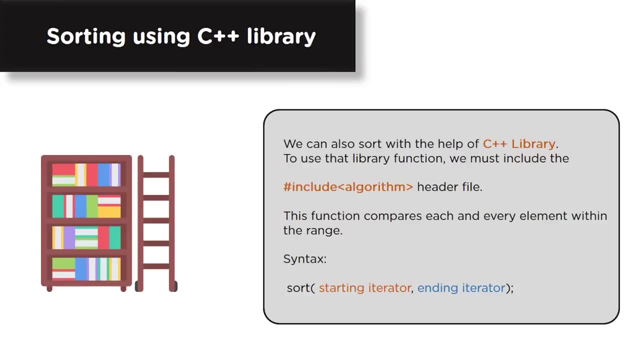 now let's understand how to sort using C++ library. We can sort using the C++ library as well. To use that library function, we must include the hash include algorithm header file. This function compares each and every element within the range. The syntax of function. 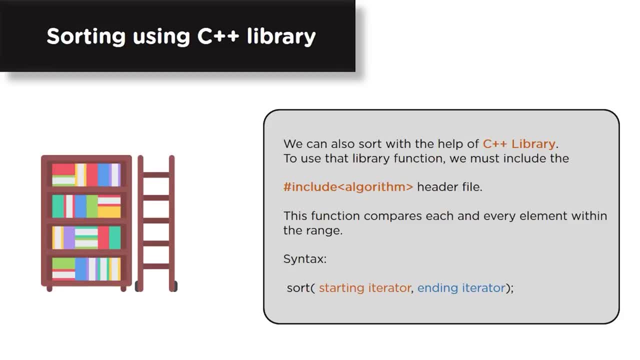 is sort, then within the brackets, there will be the starting iterator and the ending iterator And we must include this algorithm header file with hash include, which is a preprocessor. So as we have understood about these sorting algorithms, so let's move to our code editor. 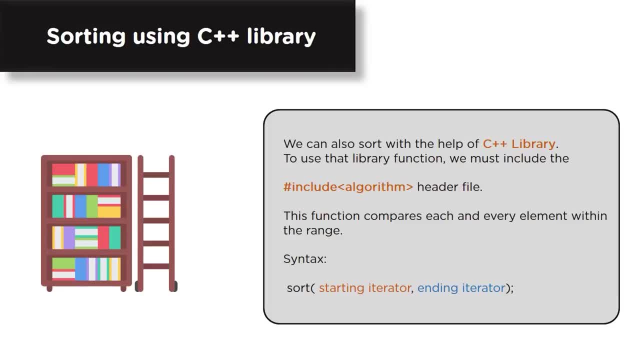 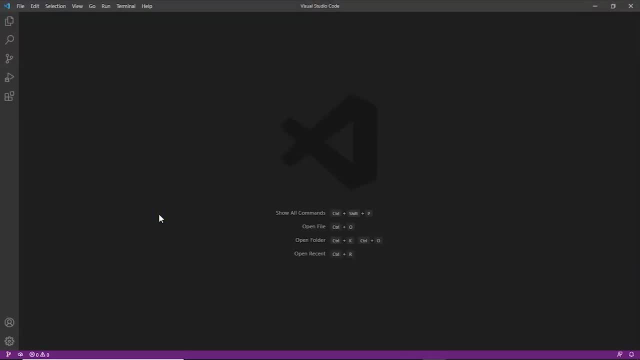 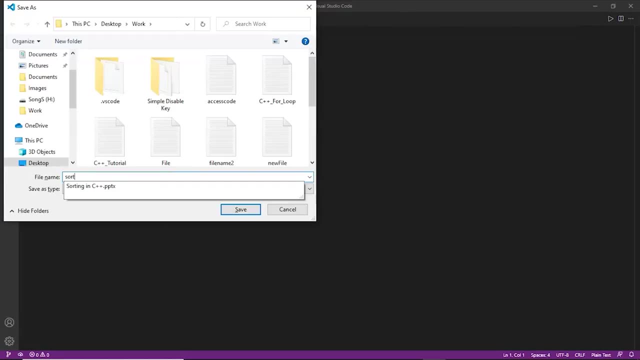 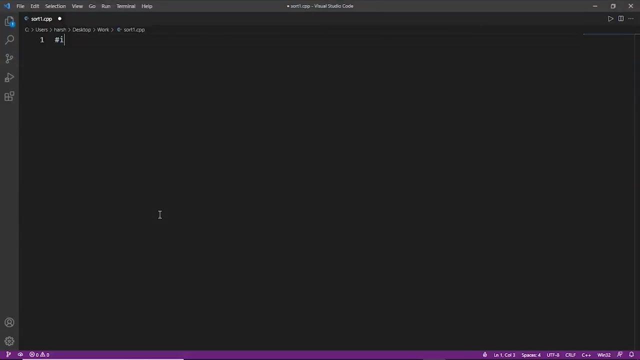 that is, VSCode, to do some examples on this: sorting algorithms. Alright, so this is our code editor and here we will do some examples of sorting techniques. So let's first of all create a new file and let's name it. So let's add first of all the header file hash, include iostream, then the namespace standard. 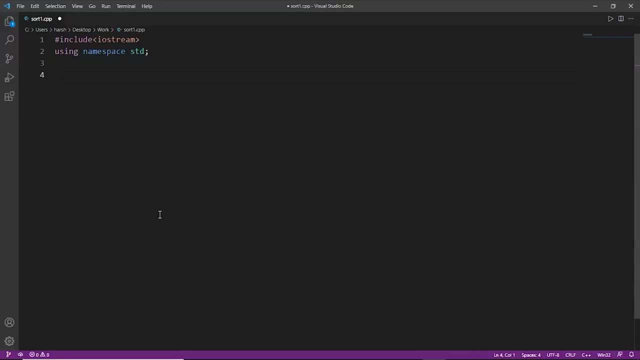 So first of all we will do an example of bubble sort algorithm and now we'll create the main function. Inside the main function, we will create some variables, let's say int i, int j and a temporary variable, temp. After that we will declare an array, arr, and let's say: 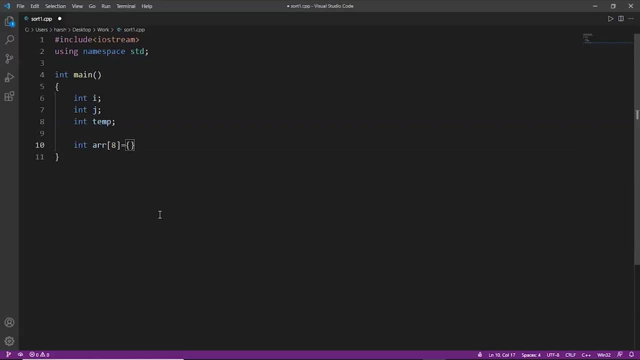 the size of the array is 8 and the elements of array are 12. let's say 3, 1,, 5,, 18,, 19,, 30.. 10, 7 and 35. so these are the elements of the array. now we will display these elements so. 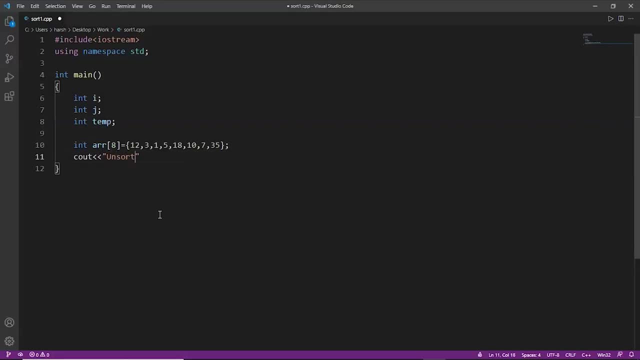 we'll display a message: unsorted array, as we know that these array elements are unsorted, so we'll print the message unsorted with slash n. all right, now we'll write the for loop: and i equals 0. that runs from i 0 to i 8, because you want to print the array i less than equal. 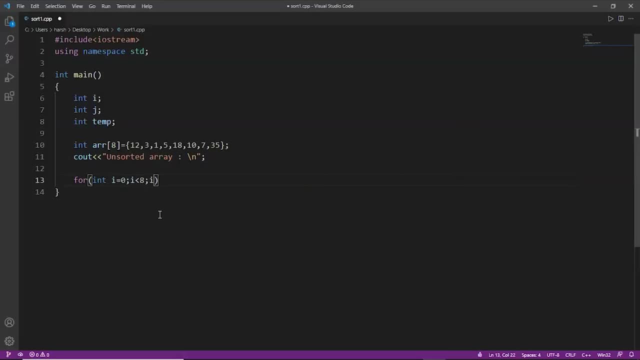 to 8, i less than 8, i plus plus. now, here we will print the array arr, i. so, one by one, all the elements will get printed and we'll add the slash t to add the horizontal space between each element. all right, now we will print the array, as we know that these elements are unsorted, so we'll display a message. 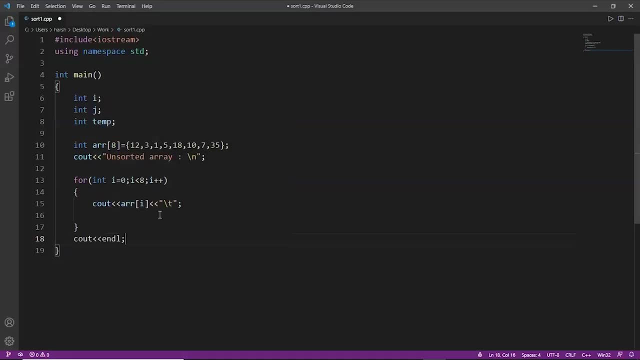 unsorted array. as we know that these elements are unsorted for space, we will write. we can write and l now we will write. led logic for bubble sort: as we know, in bubble sort the swapping is done starting from the first two elements and if the element on the left is 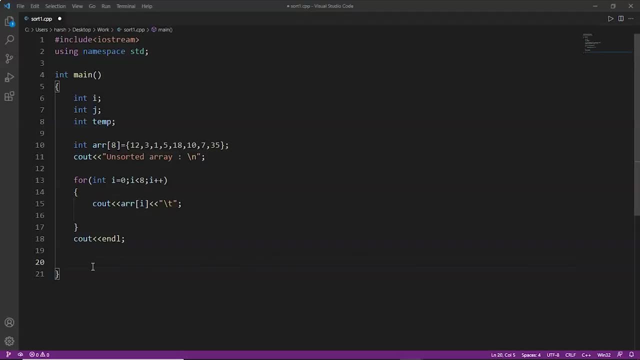 greater than the element on the right, then the swapping is done. so we will do that. we will write a for loop which runs from i 0 to 8 and i equals 0 i less than, bzw. sup wär 8 i plus plus. and the second for loop would be int. j equals i plus 1 j less than 8 j plus. 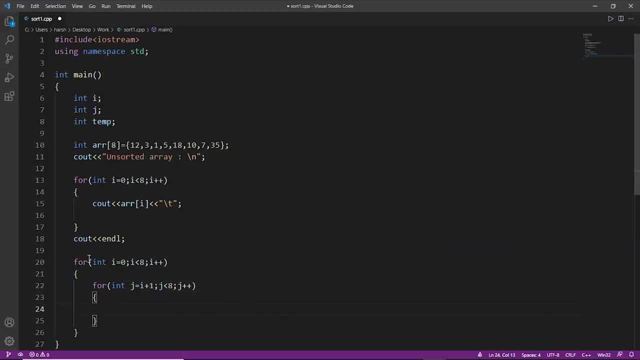 plus. now i'll explain both of these loops, but before that let us just write the if condition for swapping. if arr i is less than arr j, oh, i write the opposite of that which i have to write. let's make it i, yeah. if arr of j is less than error of pi, then we'll do the swap. so now i'll. 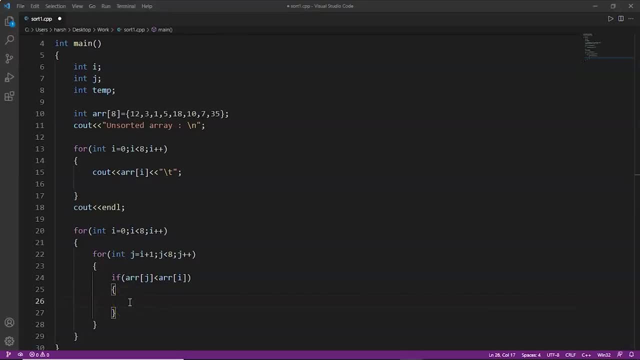 explain this part here: when i is at 0, then j is at 0 plus 1, that is at index 1. so now comparison will take place between element and index 1 and element at index 0, if the right element, that is index 1 element, is smaller than the left element, that is index 0 element. 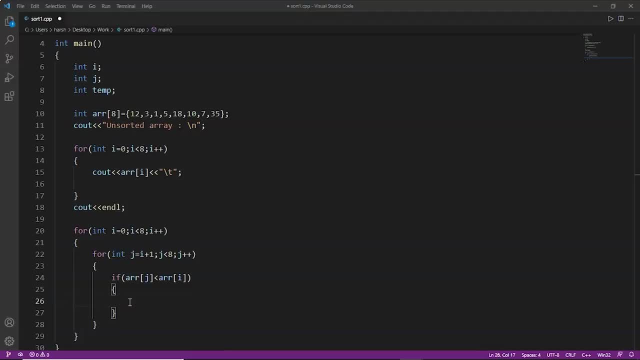 then swapping will take place and similarly, one by one, each element is compared with the next element, and it will proceed till the end of the array. so now, here we will write the swapping logic, we will store the first variable into the temporary variable and then we will store the second variable into array of i. 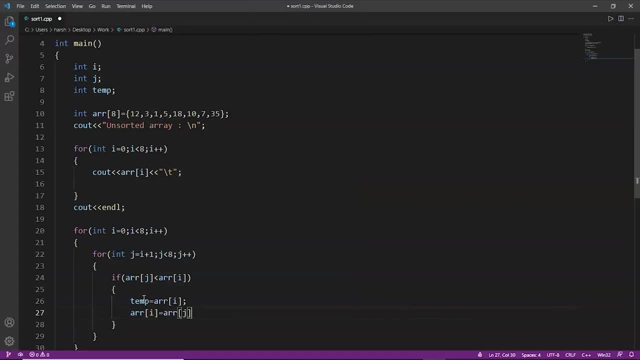 so we will store, and then we will again store into array of j the value helded by the temporary variable. all right, so this is how swapping is done. now all we need to do is to just print the array elements, because it because we have to show the 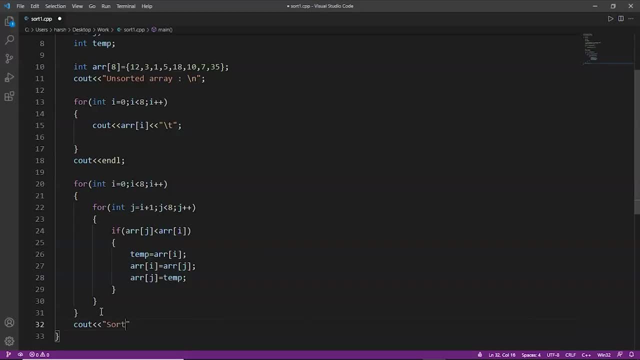 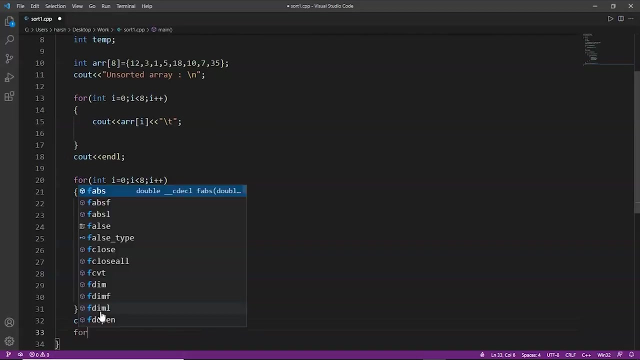 sorted elements of the array. so display a message: sorted elements. right, and then we'll use slash n as well. now, here again, we will use the for loop, and which runs from I 0 to I 8, e less than 8, I plus plus, and now we will print the elements of the array of sorted array. 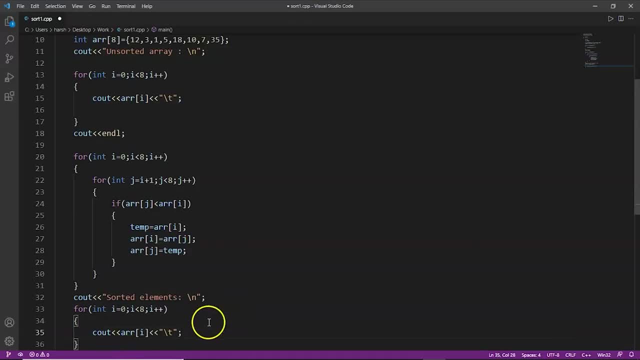 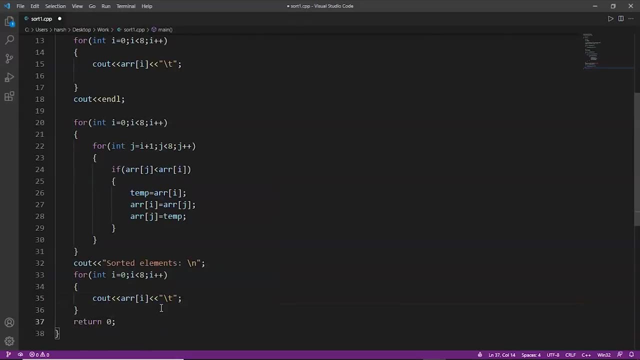 just to add the horizontal space. we can write slash T and now, after that, return 0. let's save it and let's hope it will work. so, as we can see, this is the unsorted array: 12, 3, 1, 5, 18, 10, 7, 35, and this is a. 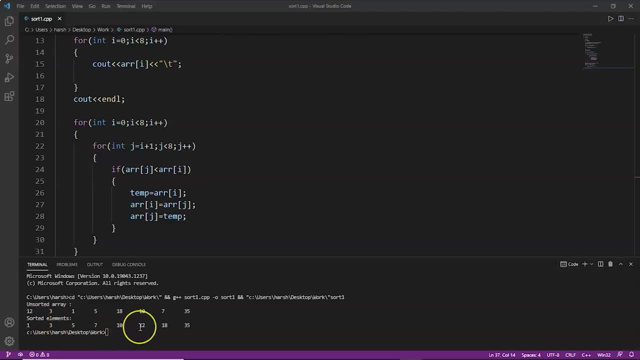 sorted elements of the array 1, 3, 5, 7, 10, 12, 18, 35. so as you can see, these elements are sorted. and using the elements of the array 1, 3, 5, 7, 10, 12, 18, 35. so, as we can see, these elements are. 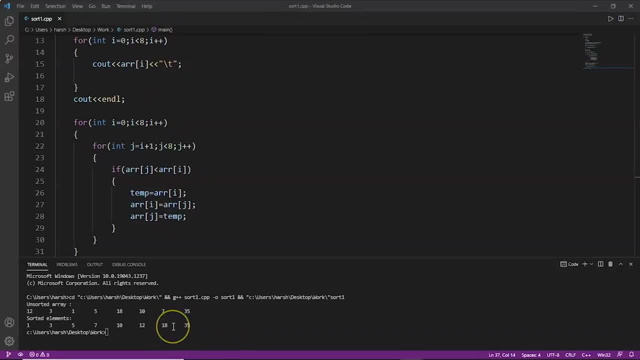 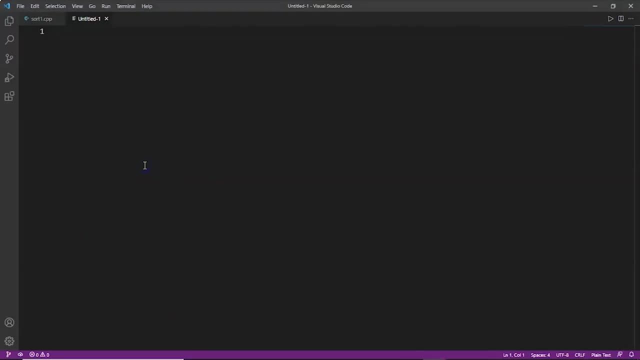 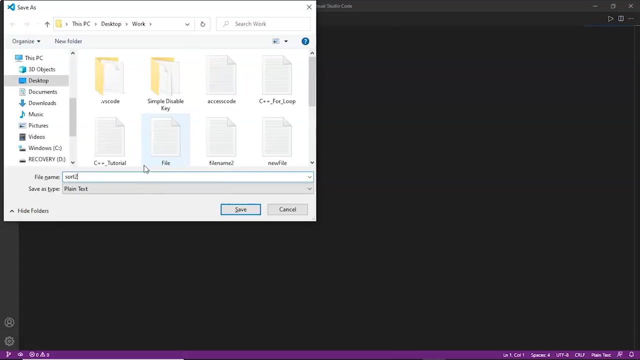 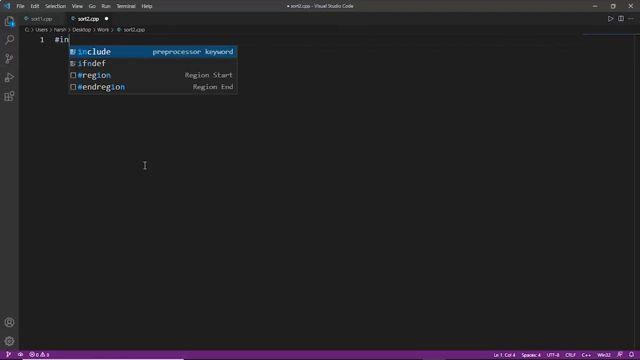 sorted and using the slash t, we have added the space between each of these elements. all right, now let's do another example. so now let's do an example of insertion sort. first of all, let's save it and let's name it as sort2.cpp. now let's add the header files hash include iostream. then write the namespace standard. 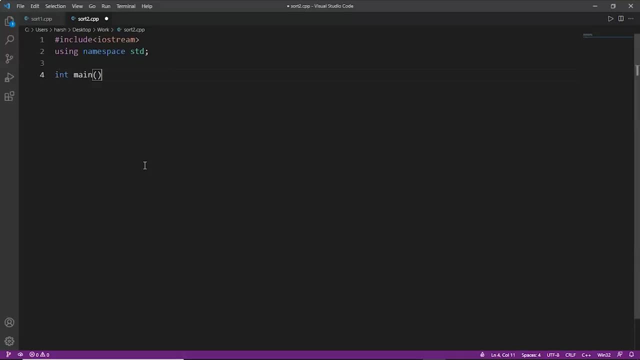 then we'll start with the main function, int main. now we'll write the variables like int i, int j and num variable, then the temp variable, temporary variable, and we'll also initialize the array. let's make it 30 size. now we'll take the input from the user, so write, enter the elements. 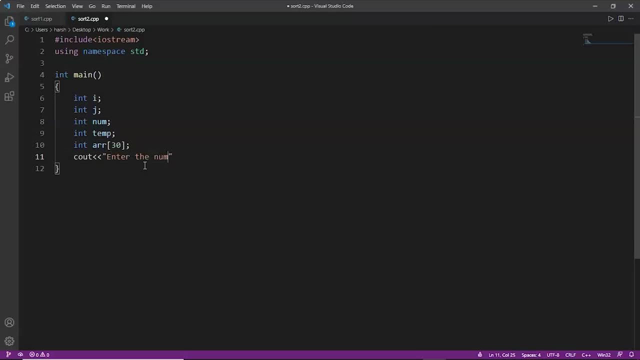 enter the number of elements first of all. all right, we'll take the input as num and then we'll ask the user to enter the elements of the array. so we'll you type expensive kind of petri, all right. all right now, using for loop of the elements of the array one by one. so num is the size of the array, so one. 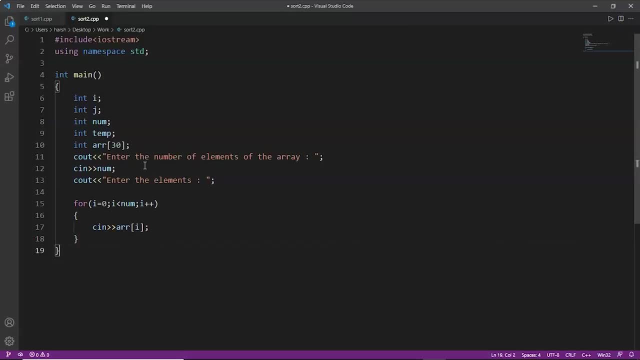 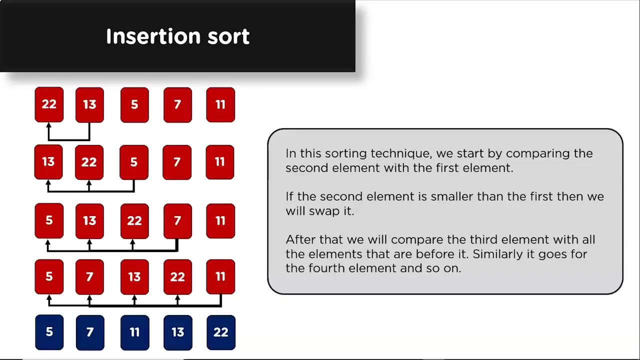 by one, all the elements will. the user will enter all the elements. all right after that. all right, now we will write the code for insertion sort. please keep in mind: in insertion sort we start by comparing the second element with the first element. if the second element is smaller than the first element, then we. 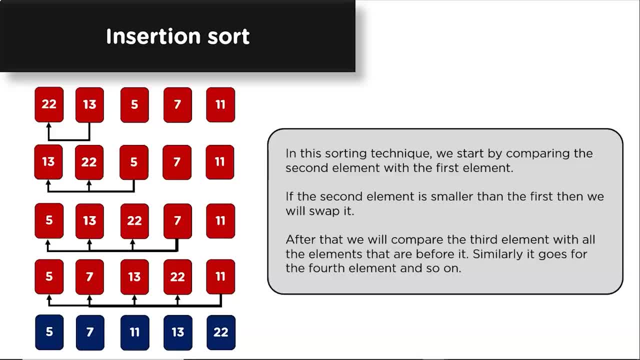 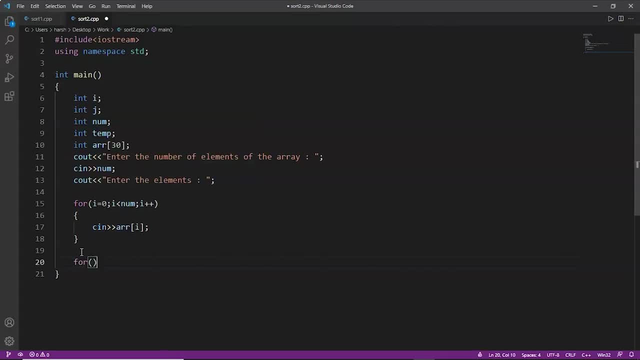 will swap it. after that, we will compare the third element with all the elements that are before it. similarly it goes for the fourth element, and so on. we can see this figure for reference, and now we'll start doing the code. we'll start by writing the for loop, which starts from 0 till num-1. 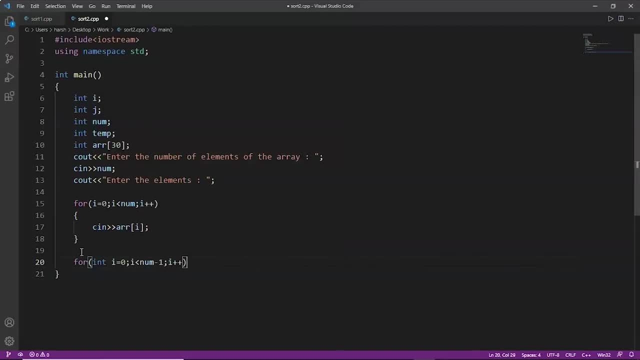 very less than them: I plus plus all right. after that we will store the array in the temporary variable. once it's done, then we'll write ji minus one. first of all we have copied the elements of array to the temp variable. then we have set j equals to i minus one, because 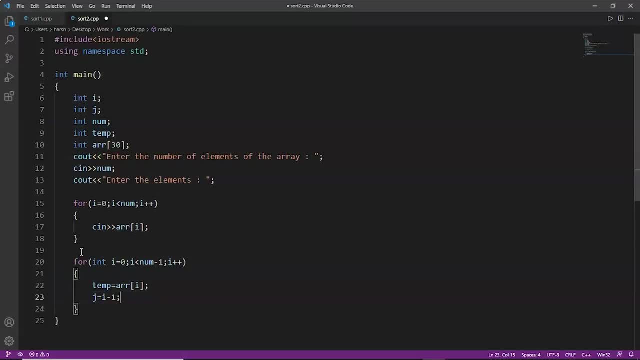 we have to compare it with the previous element, and, all right, now we will write the while loop. okay, so temp is less than ARR of J plus one, no only J. and for termination, J must be greater than zero. okay, all right, let's make them inside the brackets. 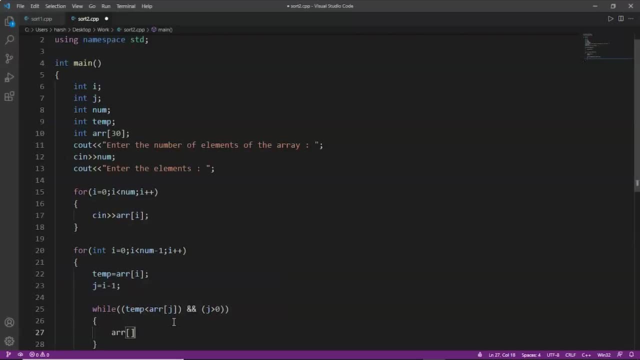 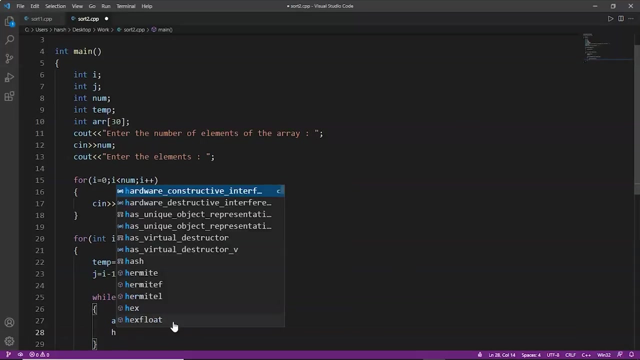 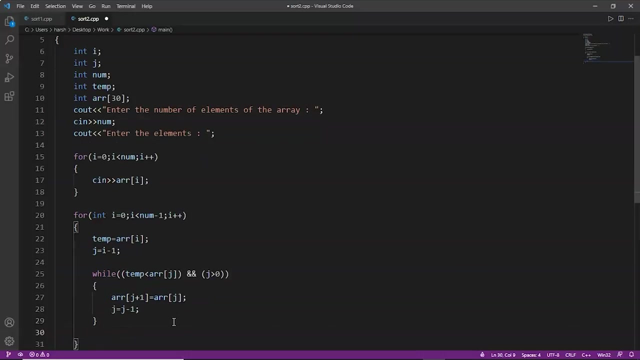 all right now. first of all, let's write the code and I'll explain the part: ARR of J plus one ARR of J. we will move this element forward and then we'll write J minus 1 willnal decrement it. then we have to insert the element in this place. 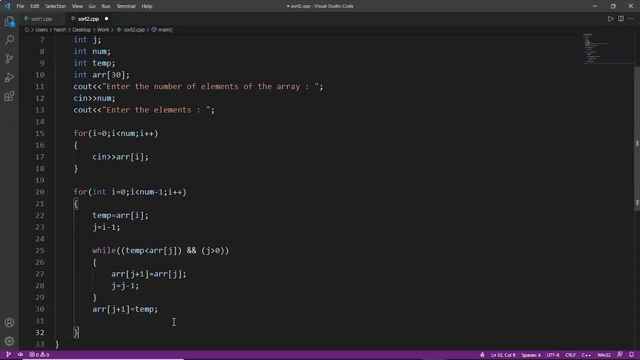 all right, I'll explain this part in this part. Okay, elements of array to the temp variable first of all, and then we have set j equals to i minus 1, because we have to compare it with one previous element and while in while loop we are checking. 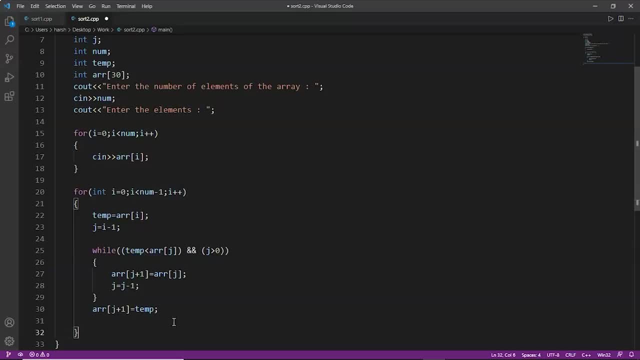 if the value of element prior to array of j is more or less. if it is less, then we moves the element in order to set it to the right position using array of j plus 1 equals to temp. we are actually inserting the element in a proper place, over the right position. we are validating that j. 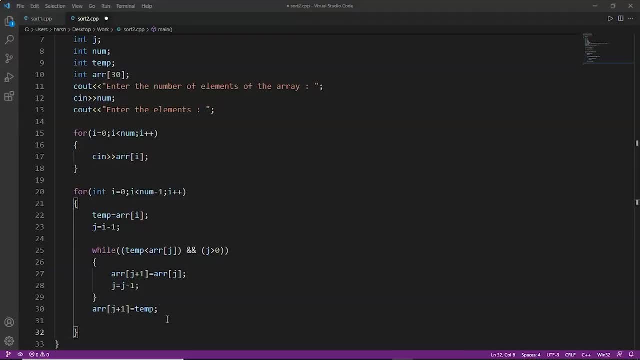 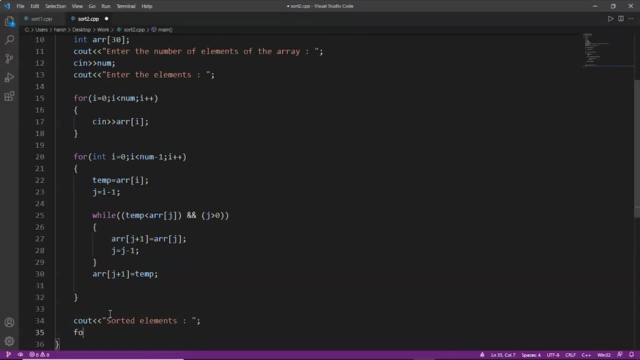 remains greater than equal to 0. so this is how it's done, and now we have to print the elements. so now we have to print the sorted element, so we will write the message, will display the message- sorted elements- and then, using the for loop, we will display all the elements one by one. 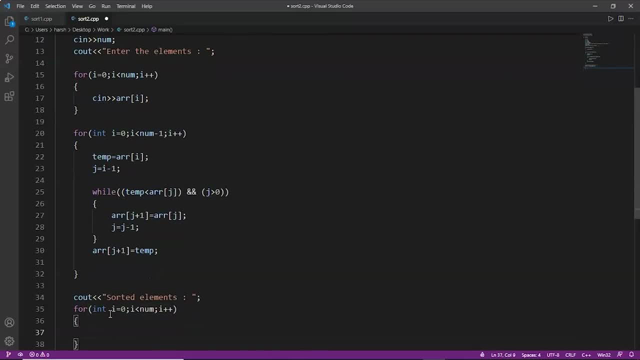 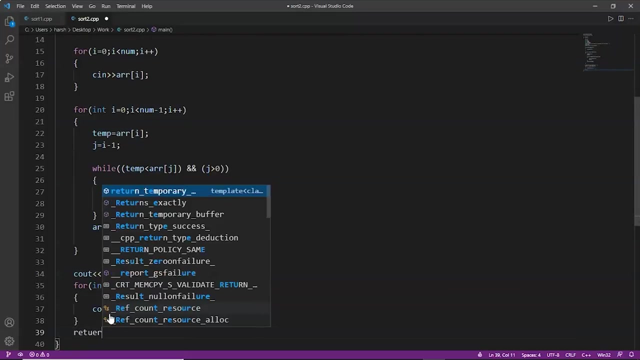 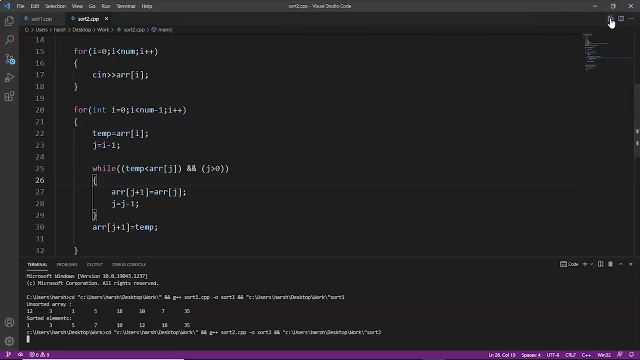 i plus plus arr. inside it will write i and we'll add some space. once it's done, then all is left is to write return zero, return zero. now let's save it. once it is saved, then now let's check if it is running fine or not. 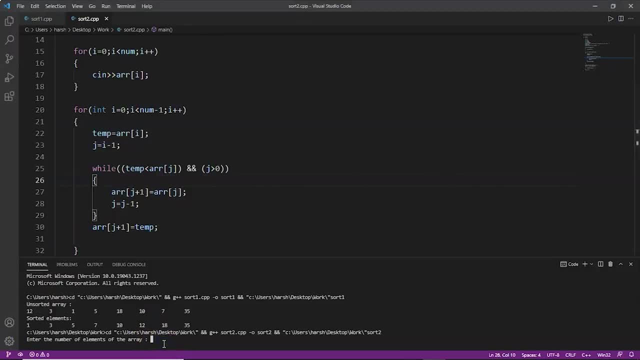 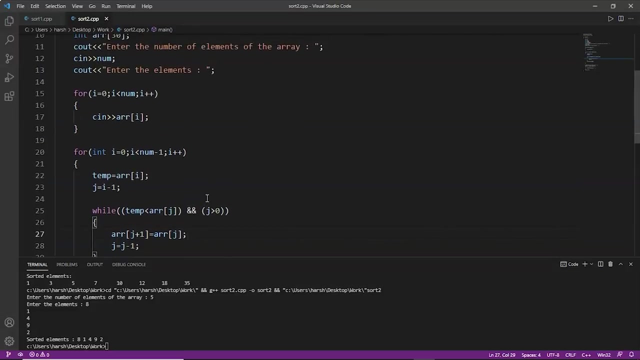 as we can see. enter the number of elements in the array. let's say there are five elements right, eight one, four, nine, two. all right, eight one, four, nine, two. so our output is wrong. let's check our output is wrong. let's check i where it is. 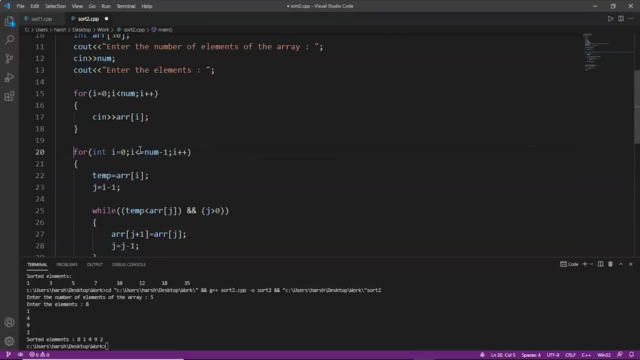 i less than equal to. this is the problem. let's save it and let's check it once more: five now. eight, five, seven, two, six, eight, two, five, six, seven. all right now, i get it. actually, we are checking from the first element, so we have to start. 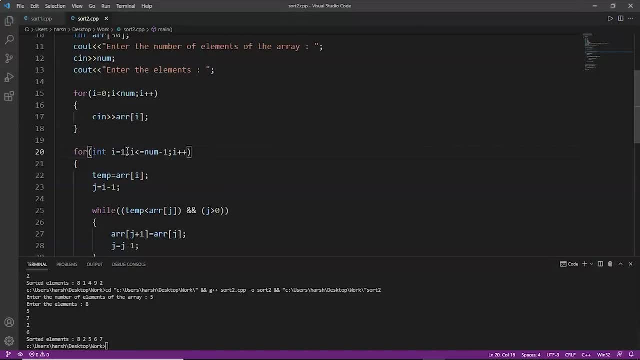 with the first index. now let's save it and try one more time: five, nine, five, eight, two, and let's say twelve, two, five, eight, nine, twelve. so finally our output is correct. because of some logical mistakes our output was getting wrong, but now we finally can see that two. 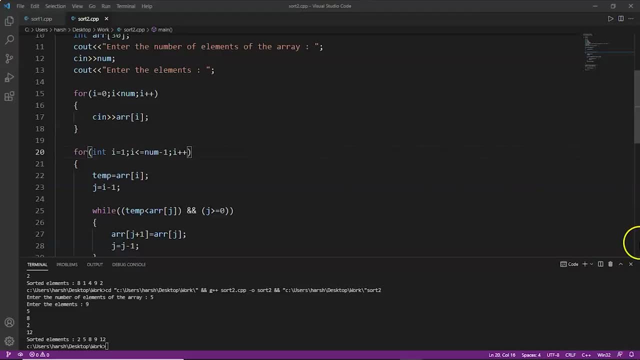 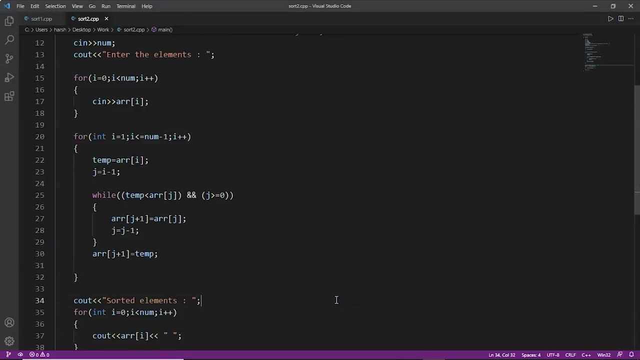 five, eight, nine, twelve, the elements of the array are finally sorted, and this is how you can do insertion sort. now, after this, we will do another example. all right, now let's do an example of selection sort. let's name it as sort three dot cbb. so let's understand. 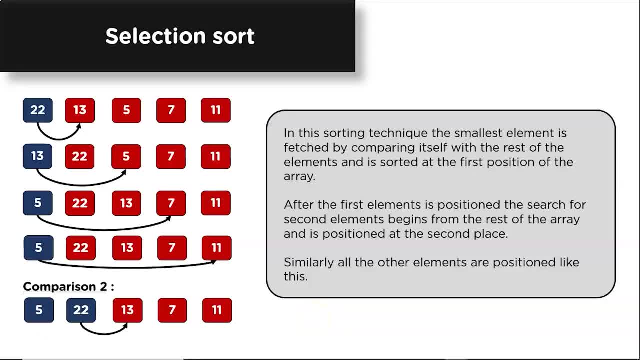 selection sorting technique. one more time. in this technique, the smallest element is fetched by comparing itself with the rest of the element and is sorted at the first position of the array. after the first element is positioned, the search for the second element begins from the rest of the array. 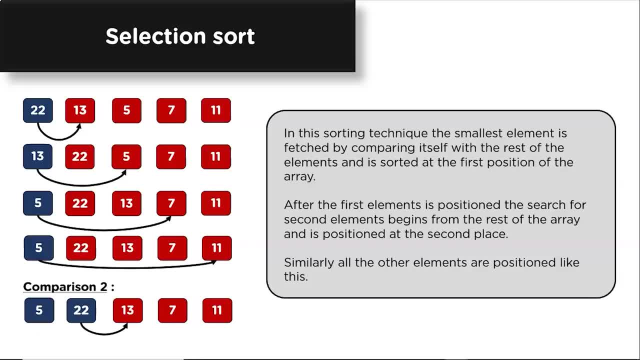 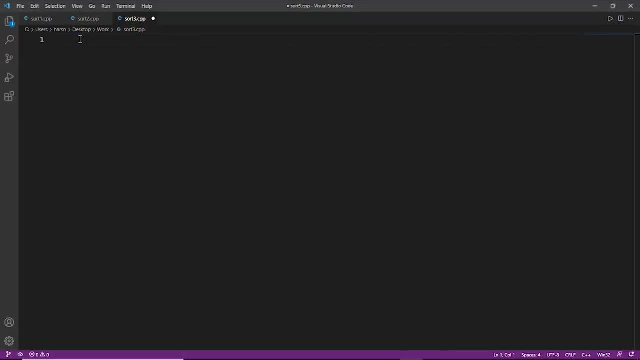 and is positioned at the second place. similarly, all other elements are positioned like this, as we can see in the figure. now let's do its practical implementation. so let's start by adding the header files hash, include iostream. then we will write the using namespace standard. now we will start with the main function. 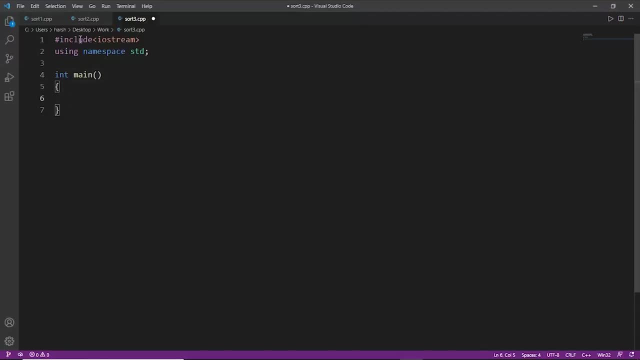 all right. so first of all we will declare some variables like int i, int, j, int, num variable, then a variable p and a temporary variable temp, and we also need a minimum variable. we will name it min. and now we will declare the array. let's make it of size 10. 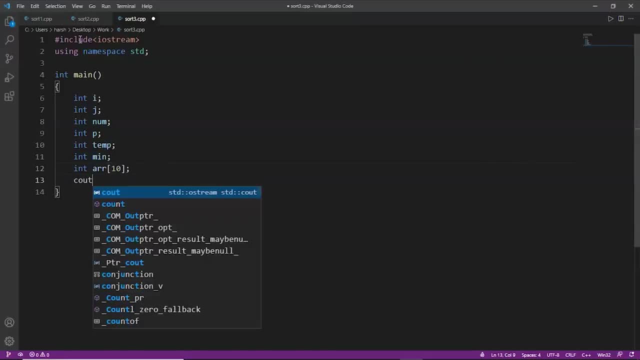 and yeah. now we will display a message saying that: enter the number of elements. we will write: enter the number of elements. all right, now we will take the input. see in num. now we will ask them to enter the elements. so we will write slash n. enter the. 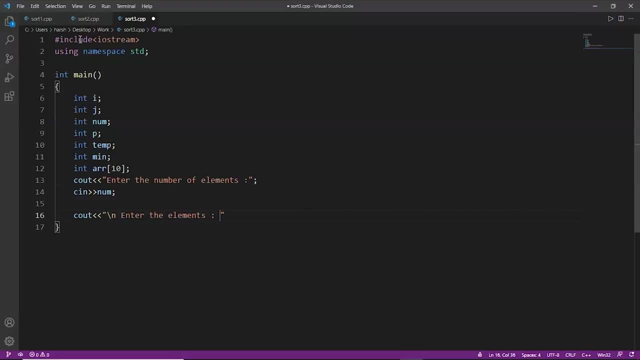 elements. all right, now again, we will use slash n once it's done. now we can take the input of the array. so we will start with int i equals 0, i less than then, num i plus plus, and now see in array arr index i. so yeah, 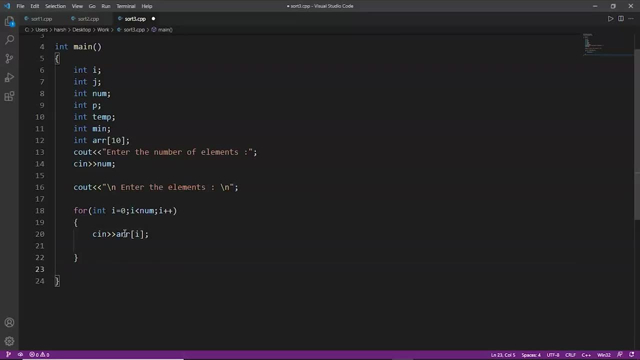 now we can take the input from the user. and now we have to do the actual part, that is, the selection sort. we have to sort the array using the selection sort technique. so let's start. we will write a for loop: int. i equals 0, i less than. 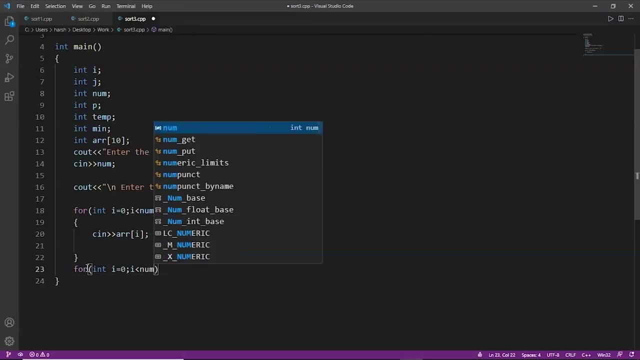 num minus 1, i plus plus. inside this loop we will store the value of the first element of the array. min equals arr of i. we are storing the first element of array into this min variable. so here we are storing the value. now we have to store the index. 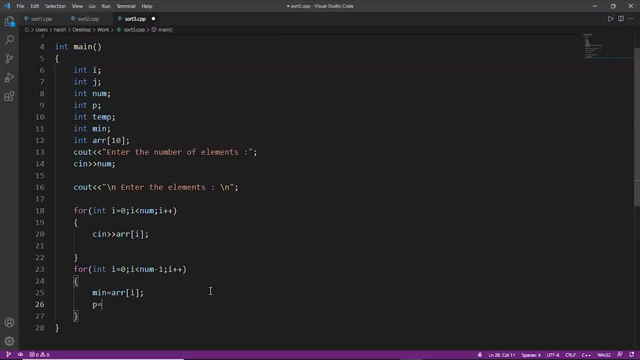 so the p variable which we have declared, and we are storing the index i to this p variable, all right. after that we have to use another for loop where the actual comparison begins. now we will write j, because to i plus 1 and j less than num. 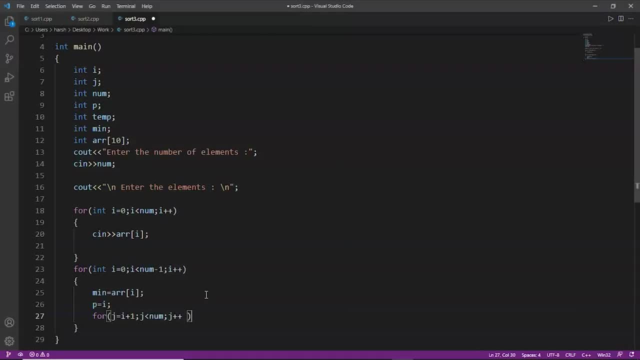 j plus plus. now i will explain you this for loop. in this for loop we are doing i plus 1, because here the comparison will take place and the comparison will occur with the preceding elements. so we have to do: j equals to i plus 1. now we have to do inside. 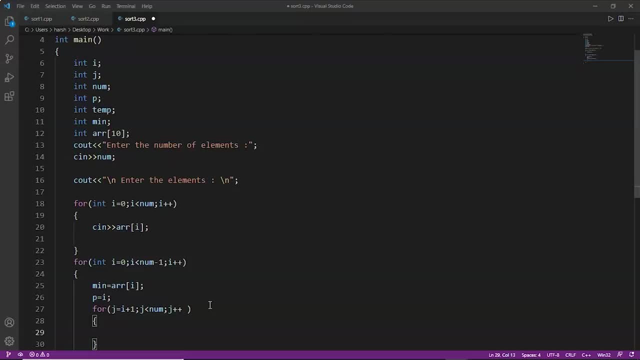 this for loop. we will use a if condition, so we will write if, if, if, if minimum is greater than array of j, that if, that is, if any element is smaller than the minimum element, then that particular element will be set as minimum element. so we will do that. 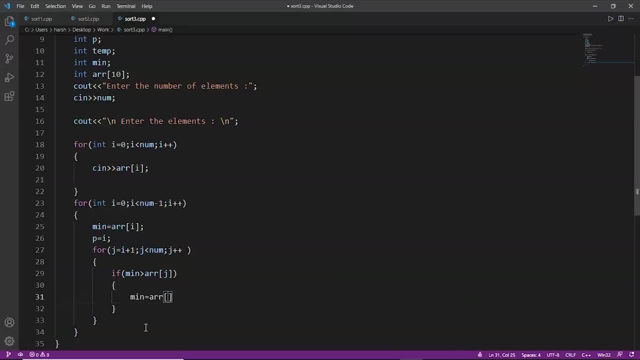 min equals array of i. array of j. sorry, and we also have to change the index. so we will assign the index of j to the p. earlier we have assigned the index i to p, but if that particular element is smaller than the minimum element, then we also have to assign the. 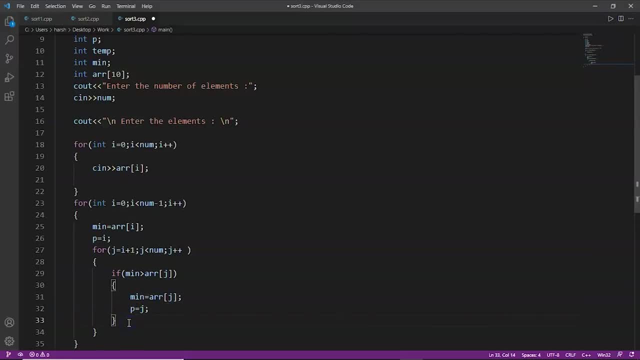 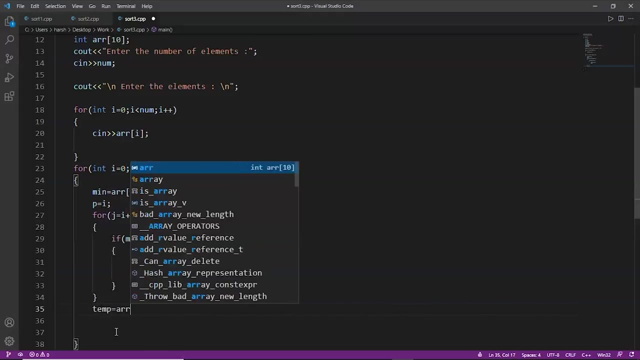 index to p. now all we need to do is to swap. so now let's do the swapping part as well. alright, so first of all, the temporary variable temp. we will assign arr of i. we have to swap arr of i and arr of p because the index j. 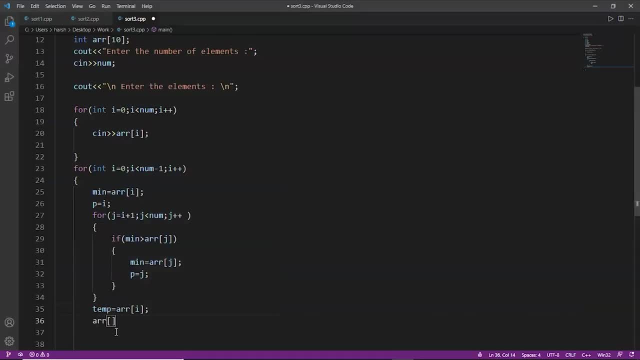 is assigned to p and we all know how to do the swapping of i. now we will put the value of arr of p into arr of i. now the value at temp goes to arr of p. so the swapping is done here and now we have to just print. 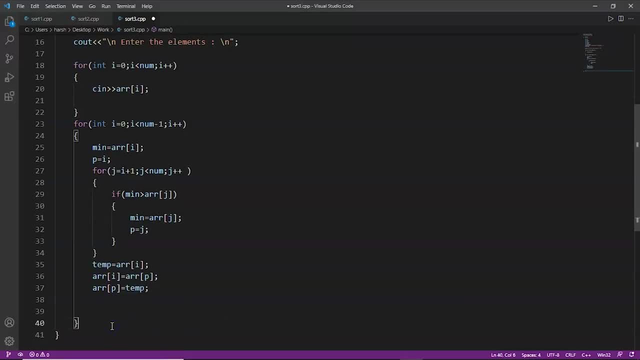 the sorted array. so now let's first of all display a message saying that the sorted elements are right: slash n. sorted elements are: slash n. again now, using for loop, we will print all those elements. equals zero. i less than n num, sorry, i plus plus. alright, now we will. 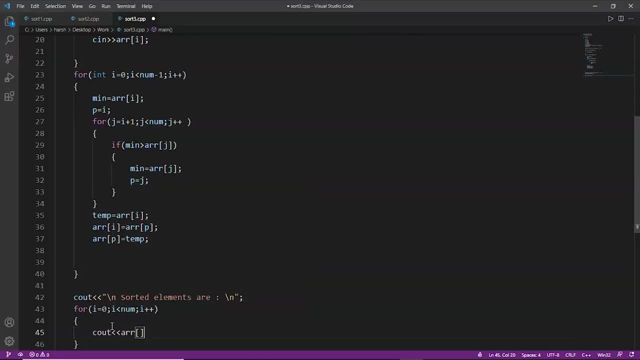 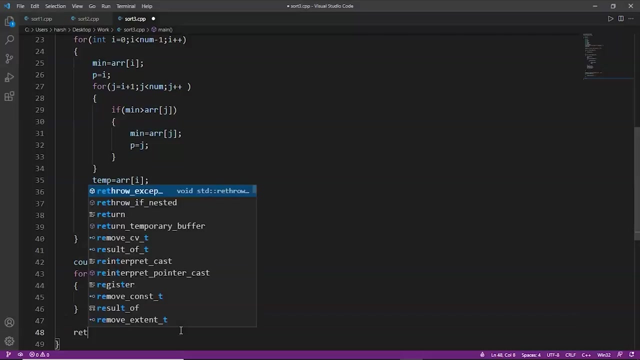 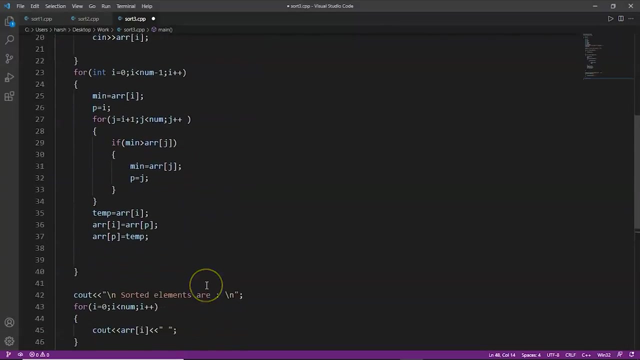 just print the array and now, in order to give some space, we will use the double quotes: now it's done. now return zero will write: now everything is done. now let's check if it is working or not. it's done by our end, so let's save it. 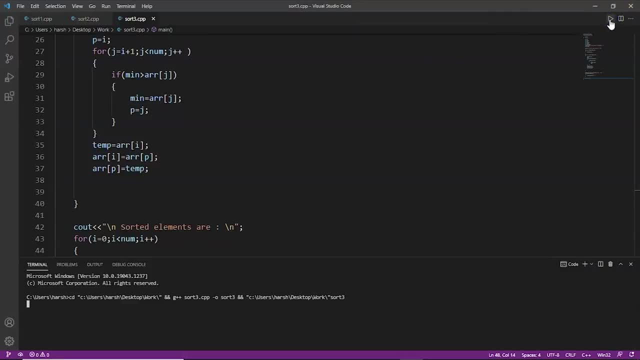 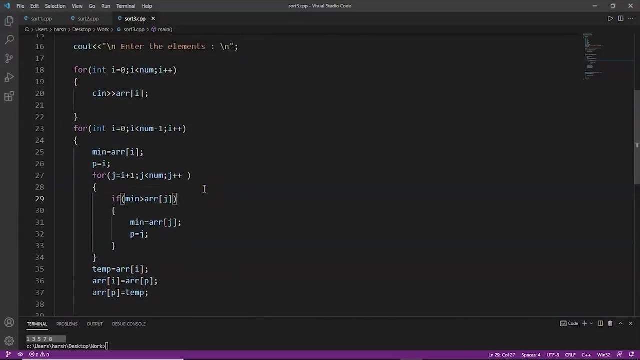 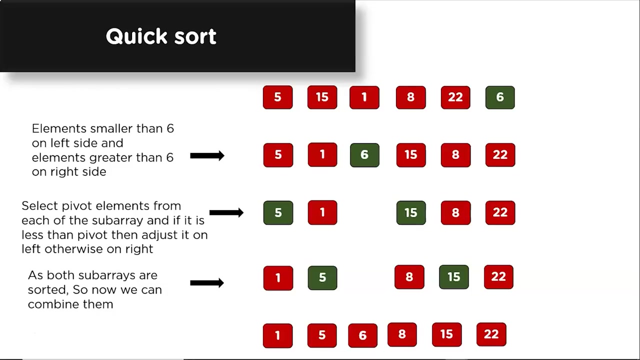 and let's try to run enter the number of elements. okay, so let's add five. now five elements are eight, one, five, sorry, one. five, three, seven. one, three, five, seven, six, six, eight, seven, seven, eight, nine, ten, fifteen, thirteen, fourteen, fifteen, sixteen, twenty, twenty twenty. the divide and conquer algorithm. so let's have a look at it. as we know in 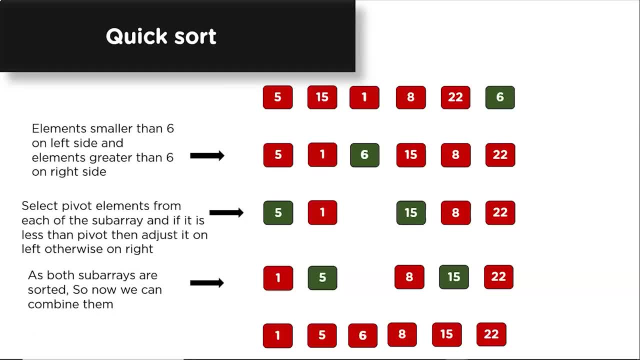 quicksort, a pivot element is selected, like here. we have selected 6 as a pivot element, and then the elements which are smaller than 6 are put on the left side and elements which are greater than 6 are shifted to the right side, and similarly, same thing is done with the partitions or the subarrays, and in the 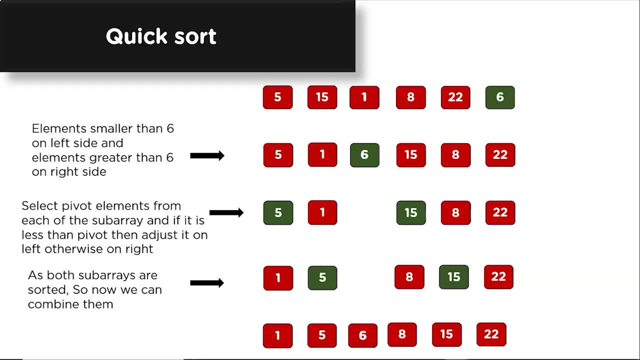 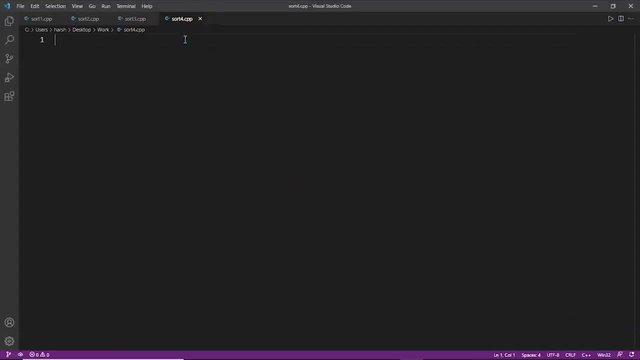 end. when we combine, we get a sorted array. so now practical implementation. so first of all, we'll start by creating a main function and before that we'll add the header files, hash, include, I've, stream and the namespace standard. all right, now we'll start with the main function. inside the main function we 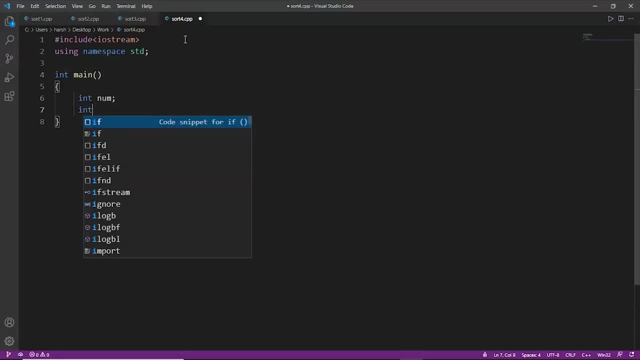 will declare a variable, variable num, and another variable, I, and declare an array- ARR to size, let's say 10. now we'll display a message saying that: enter the number of elements. enter the number of elements. all right now. here it is. now we will take the input from the user num. now we'll display: 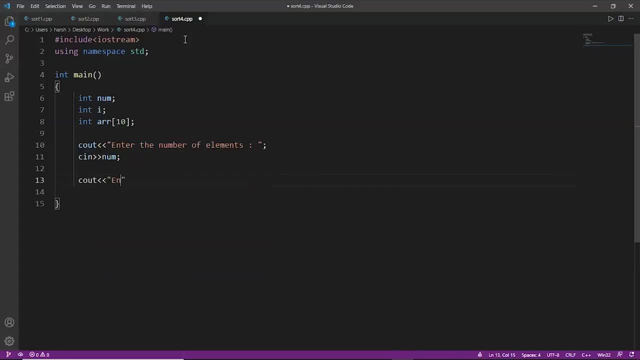 another message saying that: enter the elements. and now we'll use for loop to take the input from the user. I equals 0, I less than num, I plus plus. inside this loop, C in and ARR, I will take the input from the user. user enters all the digits or the elements. now we will call a function quick and we'll pass the arguments. 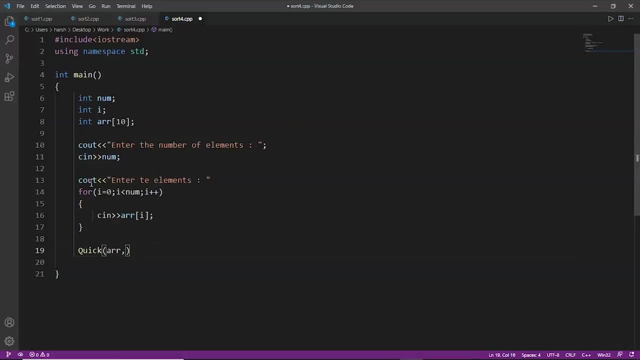 the starting index and the ending index. the starting index would be 0 and ending index would be num minus 1, that is, size minus 1. so this is where we are calling the quick function and after that we can display a message saying that, after sorting, the elements are: 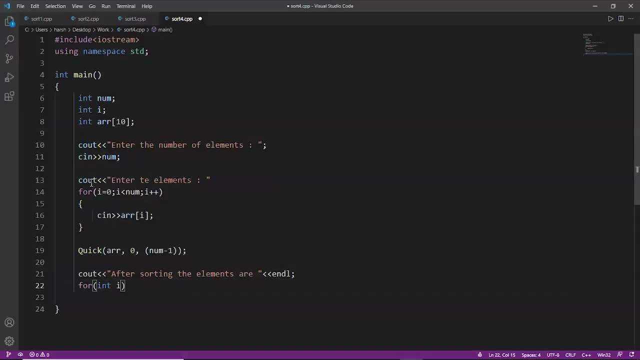 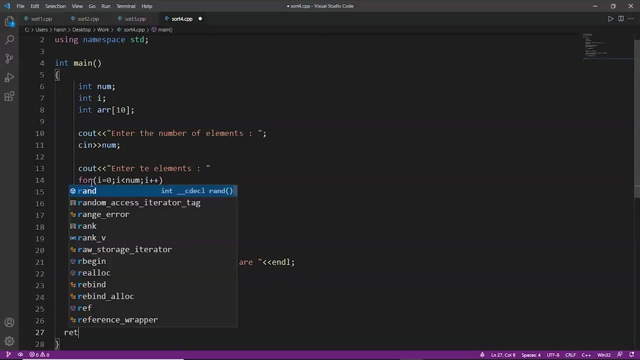 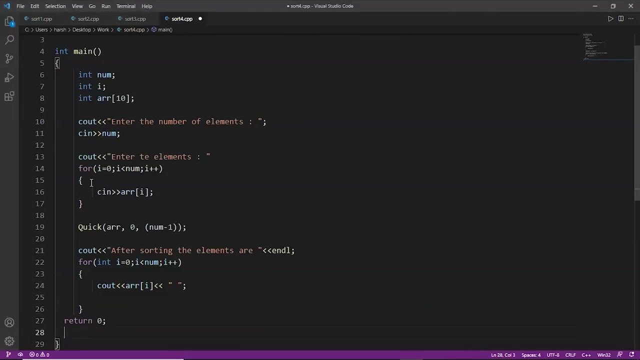 and now, using for loop again, we can display the sorted array. afterwards we'll add some space, yes, and we'll write return 0. so our main function is done. now all we need to do is to make the quick function all right. so let's create this quick function. 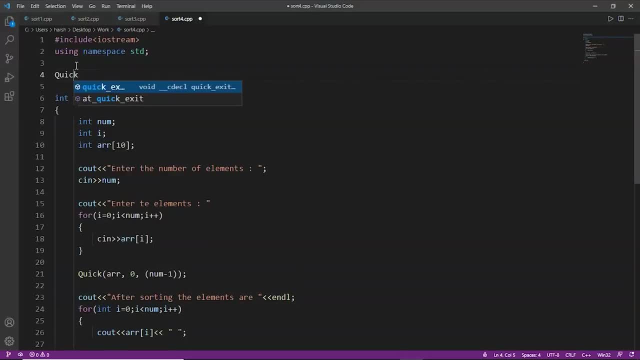 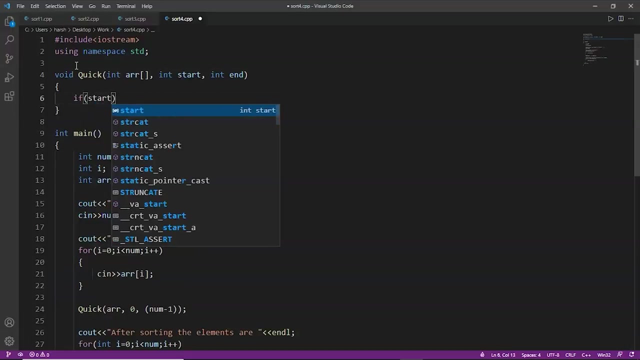 quick and its data type would be void. void quick and we'll pass the. the arguments on the parameters are array and the starting index and the ending index start int end. so these are the parameters and inside this quick function we'll write the if condition, that is, if start of the index is less than end, that is, if the array element is more than one. 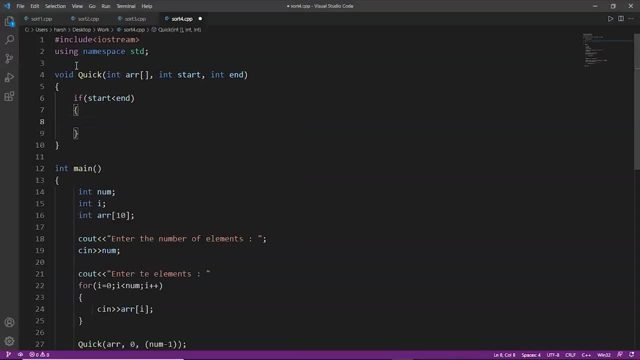 then here we will find the point of division d, and then there would be recursive calls for the divided sub-arrays or the partitions. so now we will make the division point d and now we will call om'. so now we're рядi d of x five five. so we'll divide this partinhos and the. secondary part, frente as such, and get rid of that. all right, so that's good. so now, if a function is divided, which is not true, we'll then call the, например flaps or七, and then the flaming fixed goodness named function divide and we pass the parameters array and the, the starting index and the ending index, so this function as well. so here d is the division point, and by calling this function we will end the division point. after that we will do the recursive call for the left sub array and the right sub-array. 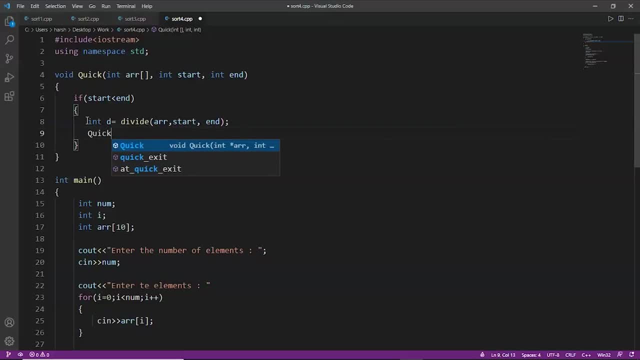 let's do that quick array in starting index and ending index. but here ending index would be as it is a sub array, as it is the left sub array, so the division point is the point of division. so the ending index for the left sub array would be: and similarly, now again we'll call for the right. 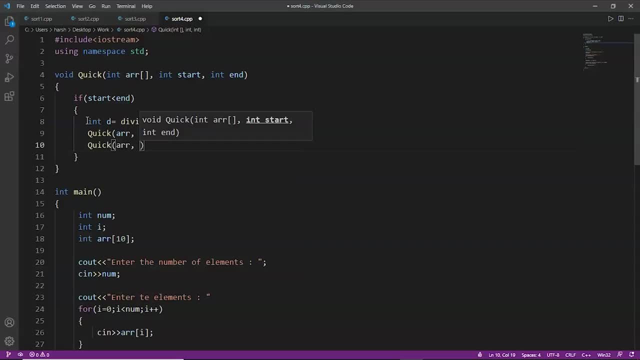 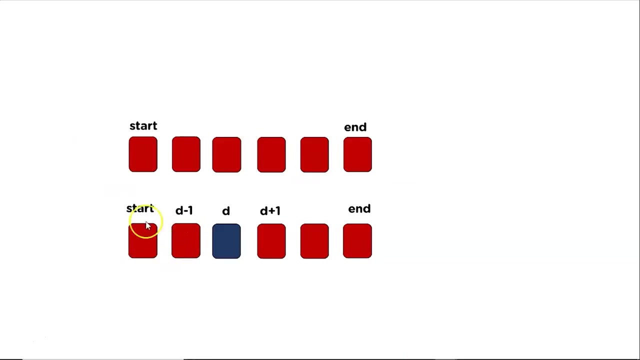 sub-array. here the starting index would be and the ending index would be. Let me explain this part again. the first recursive call would be from start to D minus 1 and the second recursive call from is from D plus 1 to the end. so these are the two. 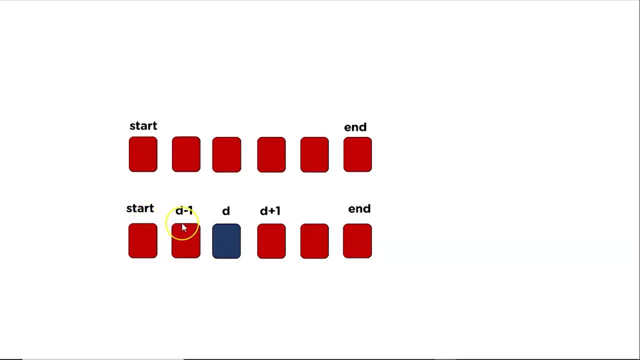 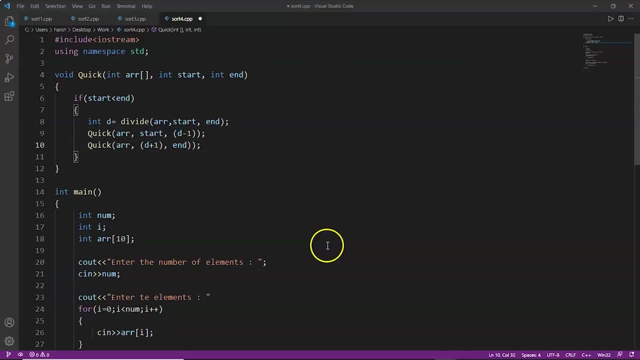 sub arrays. this is the right sub array and this one is the left sub array. so D minus 1 is this element and D plus 1 is this element. all right, now we'll make this divide function, and we have to make this divide function above the quick. 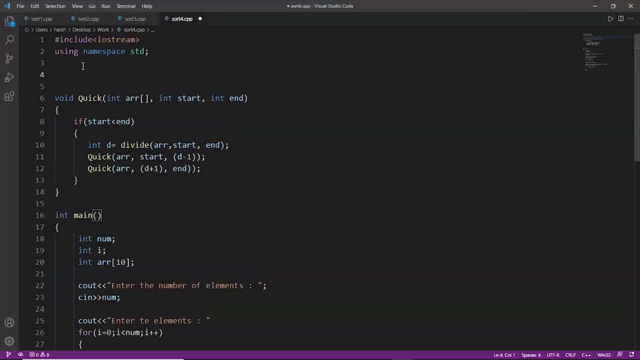 function, otherwise it will show an error. or if you don't want to do that, then you can do the forward declaration, but I'll prefer doing this only so. int is the data type, divide is the name, and now int arr, as we have passed the starting index and 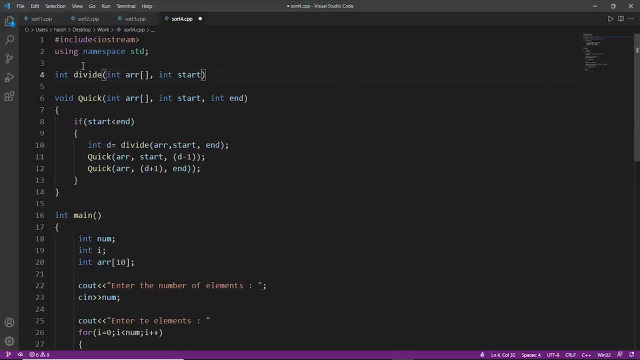 sorry, the starting index and the ending index all right now inside this divide function. first of all, we will set a pivot element. so we'll do that, arr we always. we usually select the last element as pivot element, or you can select the first element as well, or any random element. now, 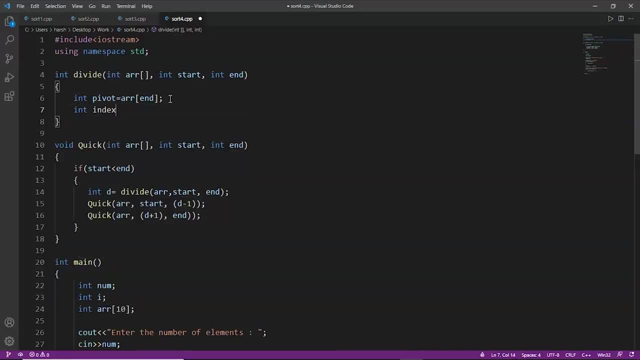 we'll create another variable, int index, and we'll assign it start index. now this variable will keep the track of elements in the array, starting from all first element and all these elements. so now we'll use a for loop and now we will do the comparison with the pivot element. so inside the for loop, int i equals zero. 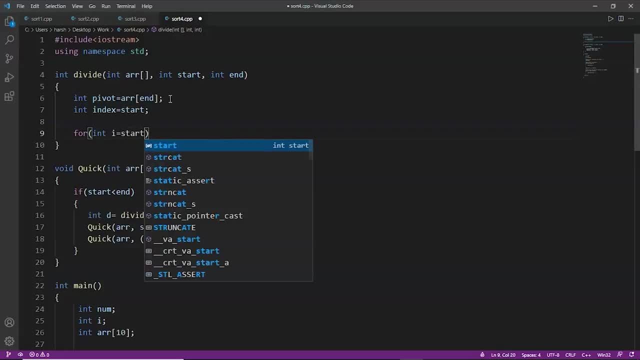 sorry, int. i equals zero, sorry, I equals start, because we'll start from the first element. So I equals start. I less than, and we will not use less than equal to. we'll use I less than n because we don't want to include the pivot element, So that is why we'll use I less than n, and now I plus plus. 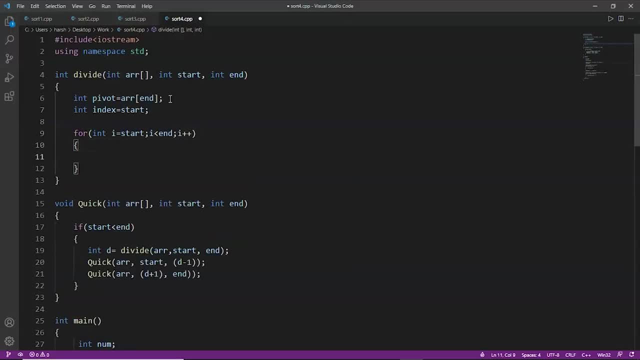 Alright, now inside this for loop we will create if condition. Now, in this condition, if the array of I is less than the pivot element, then we will shift it towards the left, then we'll do the swapping. ARRI is less than pivot, then temporary variable temp. And we all know. 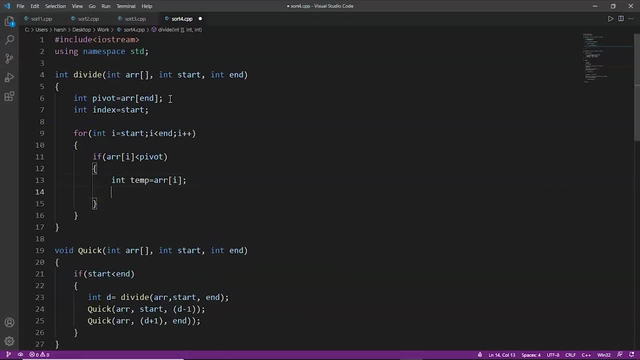 how to do the swapping. So we'll do that. ARRI index. please note that index is storing the start and pivot is storing the end. So keep in mind that now ARRI index, this temporary variable, Now we will increment this index. 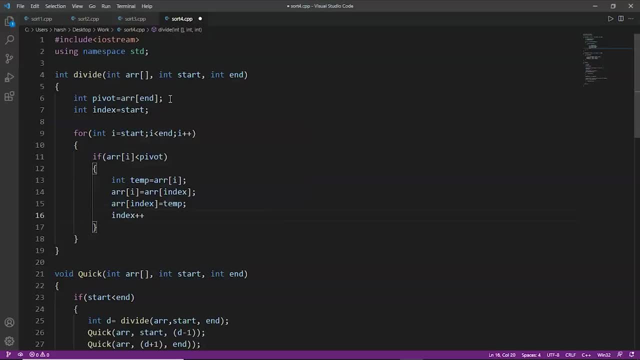 plus plus, because this index plus plus will do the further computation. And now we will look at the pivot element. So if that particular element is smaller than the pivot element, then it will move to the left side, otherwise on the right side All. 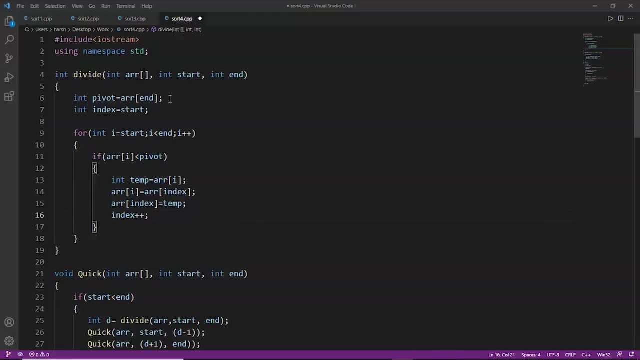 right now. it's done. Now the only thing left is the positioning of the pivot element. And to do that, because we have to find the partitioning point, So we have to position the pivot element at its proper place. So for that we'll use the temporary variable. 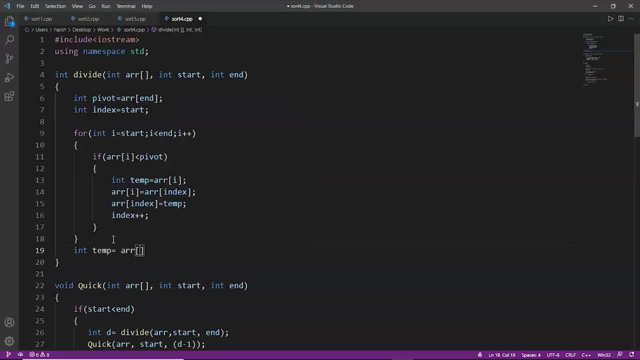 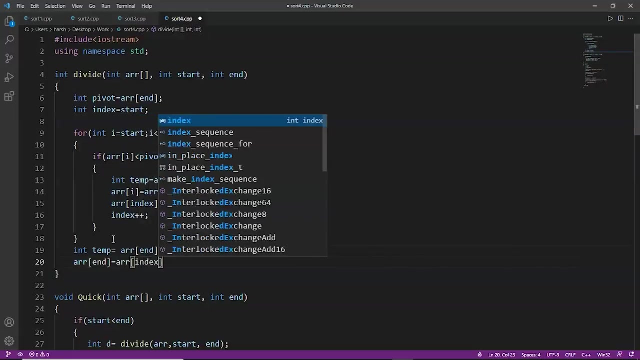 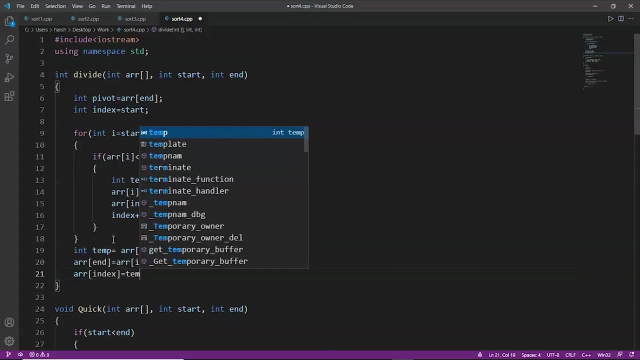 again and ARR and index. then we'll swap it with index. so here we are done with the swapping. Now we have found the partitioning point, So we'll return the index. Now the pivot is at its proper position. Now all the elements on the left side of the pivot element are smaller than that and all 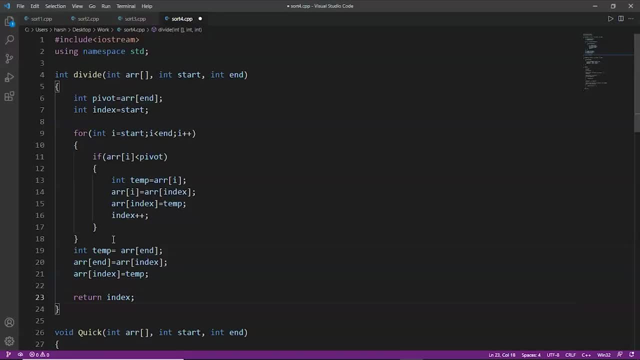 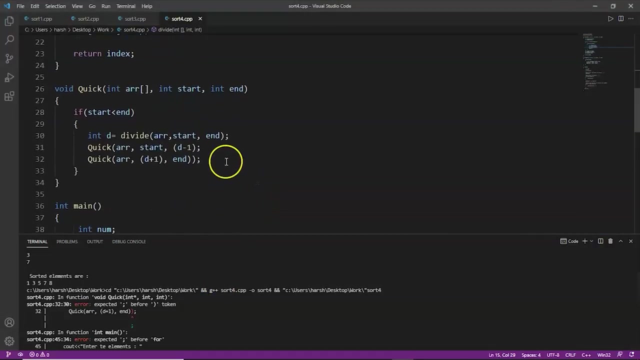 the elements on the right side of it are greater than that. Now let's try to save it and run it. I hope it works. There are some errors? let's check, alright. alright, let's do it, And this one is. this one is extra.